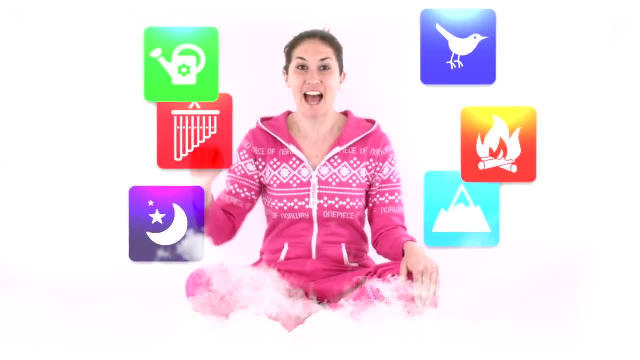 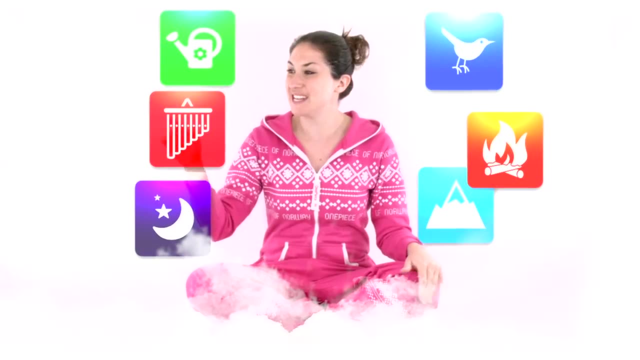 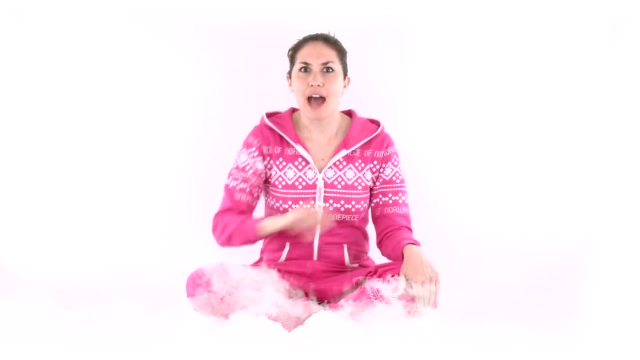 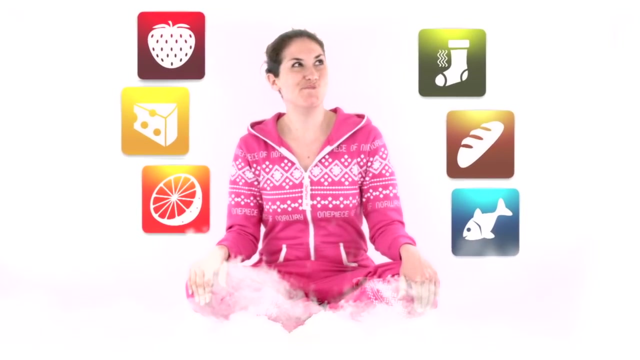 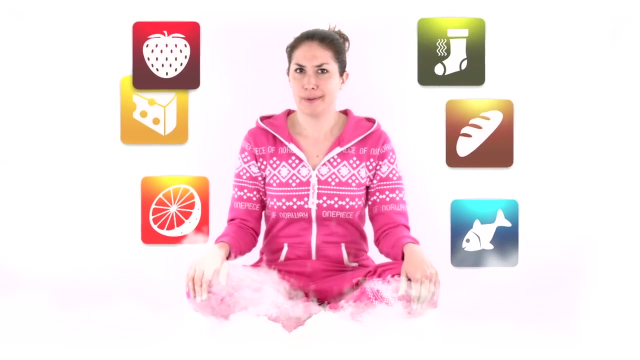 The sound of a garden, Birds in the trees And twinkling chimes in the breeze- Lovely. Now what about smell? Let's see what we've got here. Mmm, look at all these. I'm not sure about the cheese or that smelly sock, Let's go for. 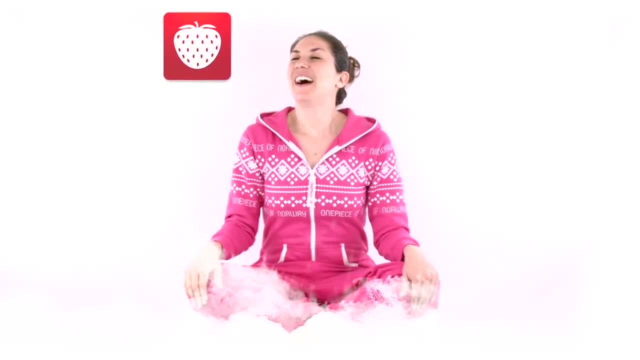 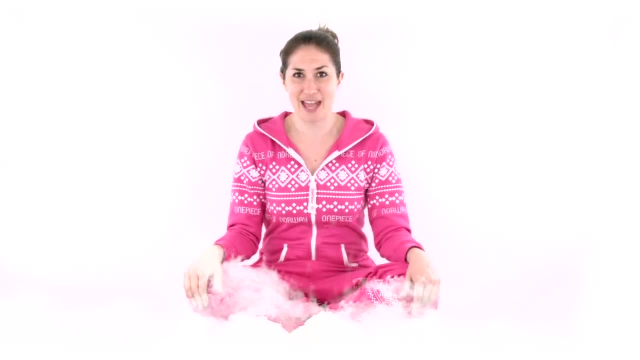 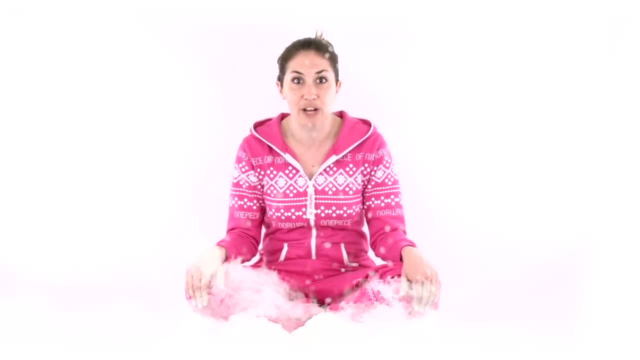 And we can't think clearly. Can you see all the stuff clouding up our heads? The snowflakes are like our thoughts, flying around in all directions. We need to settle the snowstorm with our secret trick: Our breathing Ready. Let's see if we can calm this snowstorm down. 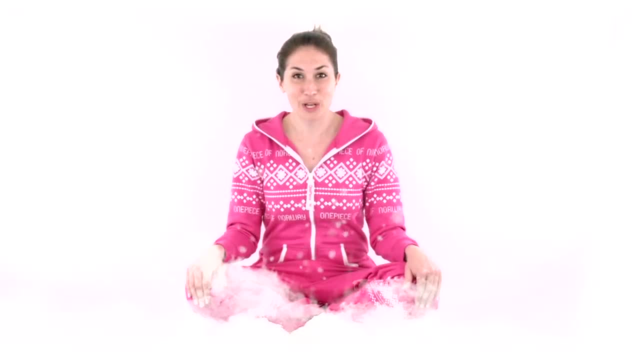 We sit nice and still Can you close your eyes and tune in to all this? all those pretty sounds, Wow. We can maybe hear some other sounds too, And if we're very quiet and we listen very carefully, we can maybe hear our own breathing. Yes, we can. 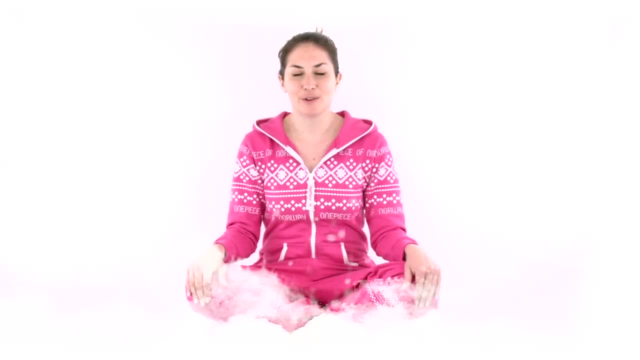 We can slow it right down and breathe, Listening to it going all the way in and all the way out. All the way in, All the way out. That's it. The snowstorm is starting to settle. You're doing really well. Let's keep going All the way in, All the way out. Last time, All